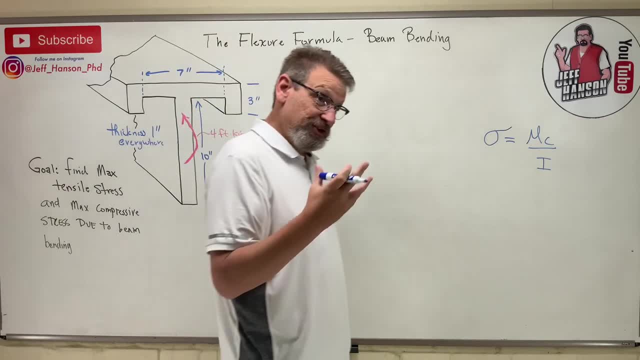 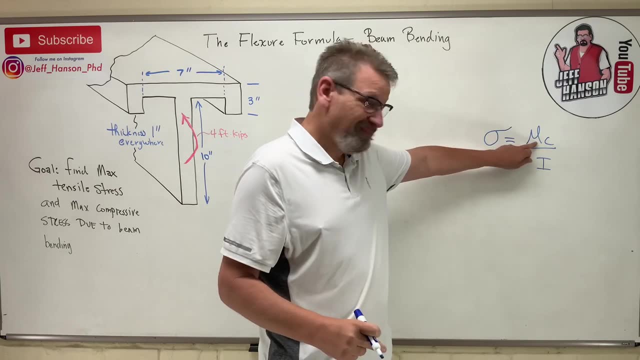 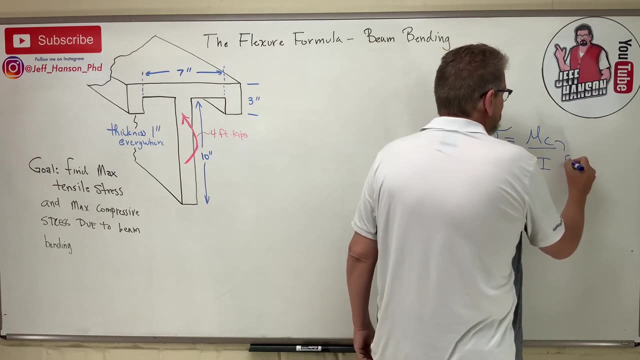 shear moment diagrams. Well, that shear moment diagram is how we're going to find out what that bending moment is is on the beam. So m is the bending moment that we know c. what is c? c is just the distance, And it's the distance from the neutral axis to the point of interest, the poi right. So it's. 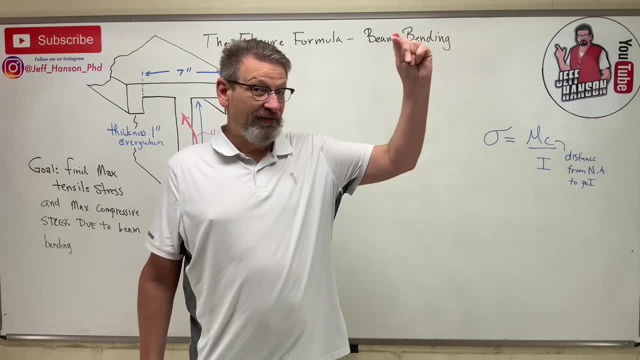 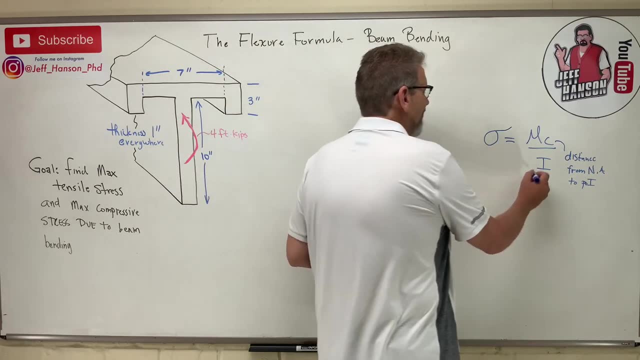 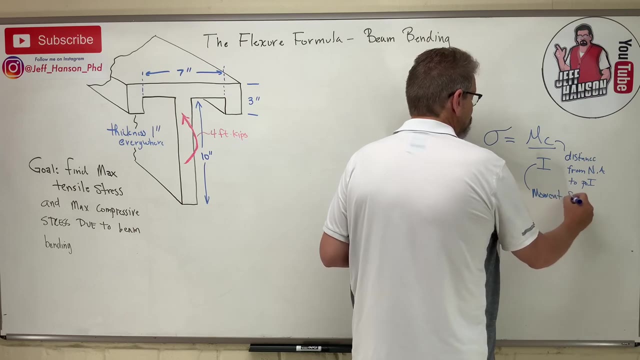 the distance from the neutral axis of the whole beam to the point of interest that you're interested in finding the stress at. So I can find the stress anywhere on the beam, okay. And then of course i i is the moment of inertia. okay, The second area moment. 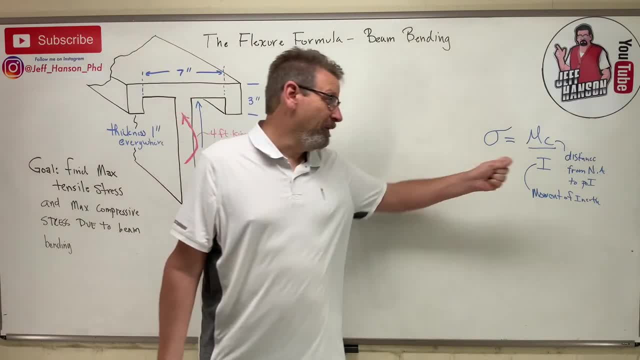 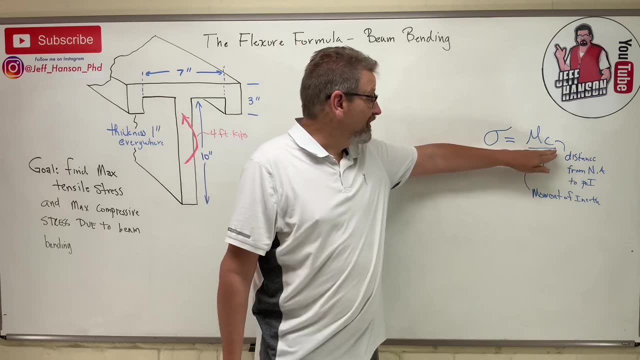 of inertia, which we learned to calculate way back in statics. If you don't remember how to calculate, i go back to the statics lessons and review that. It's the last ones we covered in there, So here's a question for you. What would be the stress in a beam due to bending? at the neutral axis. Well, the distance from the neutral axis to the point of interest would be zero. So at the neutral axis there is zero stress in the beam, So the stress only occurs the. the biggest stress occurs at the outside of the beam, as far away as you can get from. 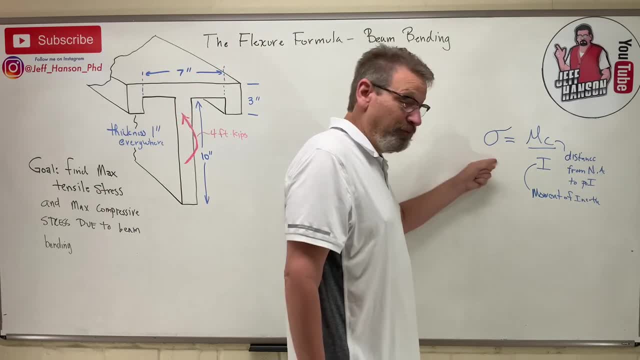 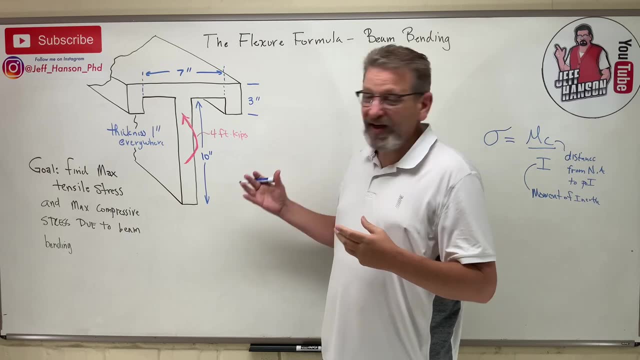 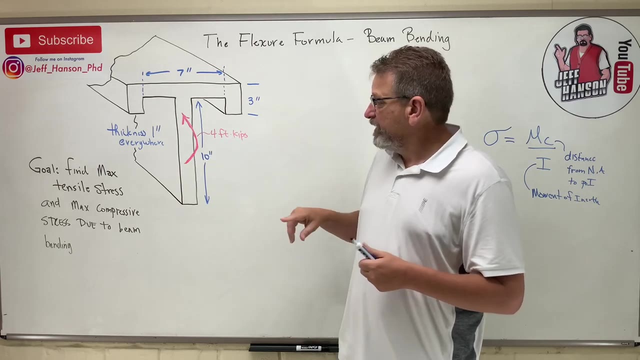 the neutral axis. So let's see how we use this formula, the flexure formula, to solve this problem. Now this one: i don't have to do, um, i don't have to do a bending moment diagram, because m the moment is just flat out given on this one, okay. so one of the things i want to just 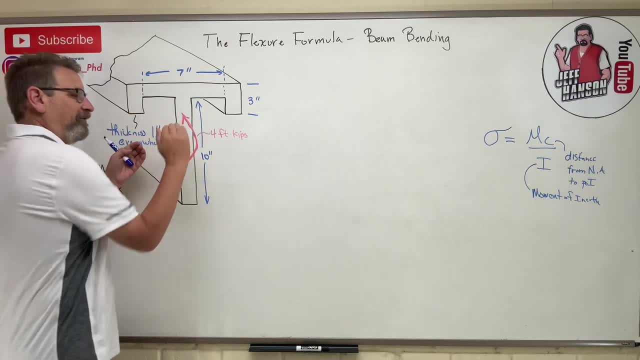 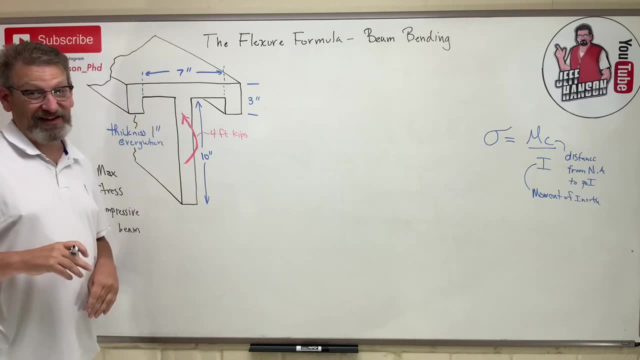 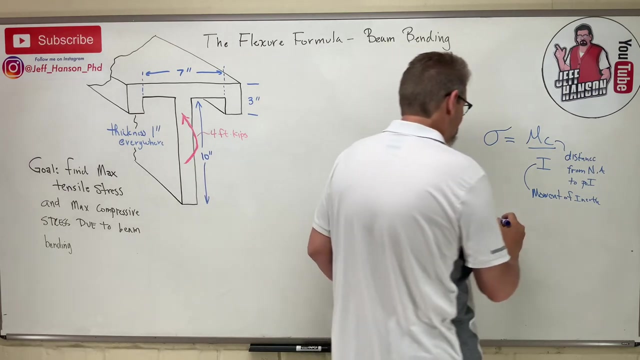 initially think about is if this is the beam. if i put that kind of moment on there, do you think the top is going to be in compression or tension? i think it's going to be in compression too, and the bottom is going to be in tension. now stress is going to have a sign. okay, so for sigma tension. 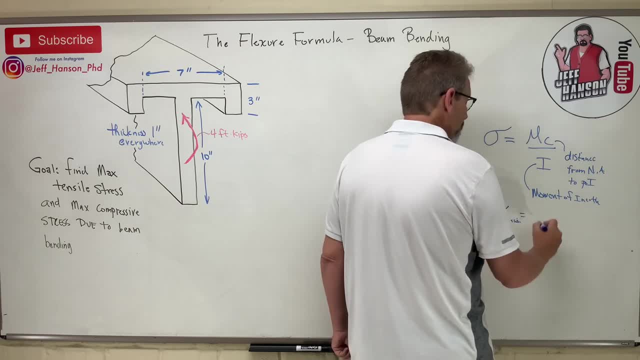 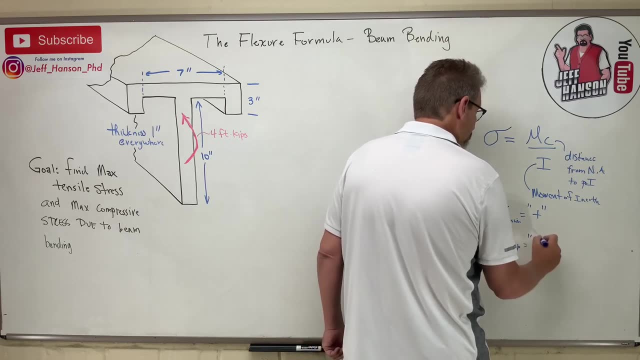 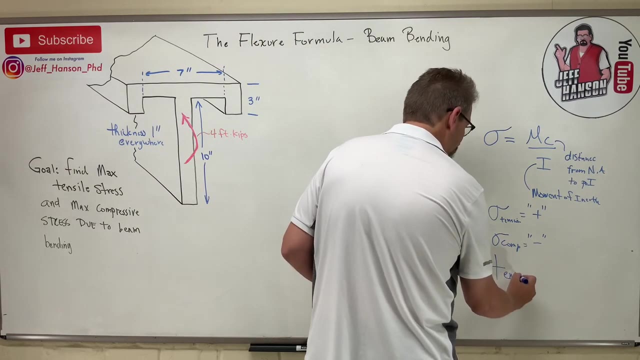 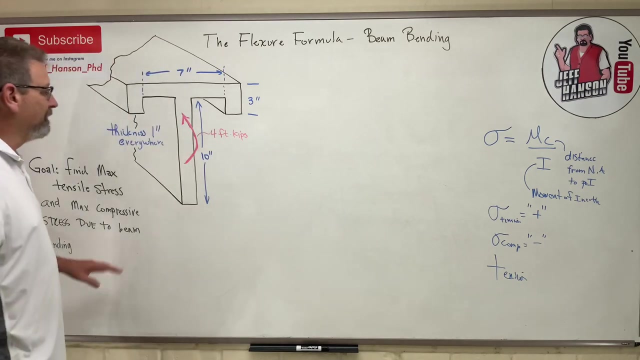 it's going to be a positive value. okay, for sigma compression you're going to have a negative value. how do i remember that? it's easy. what does tension start with a positive sign? okay, all right, that's silly, but hey, it works, man. okay. so here we go, step one step. 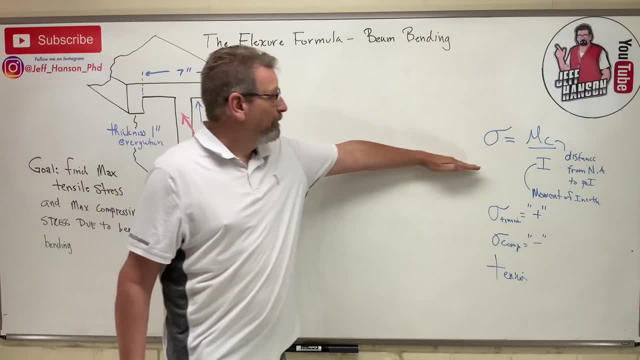 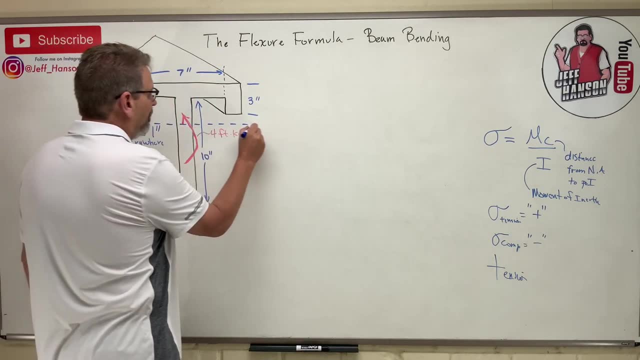 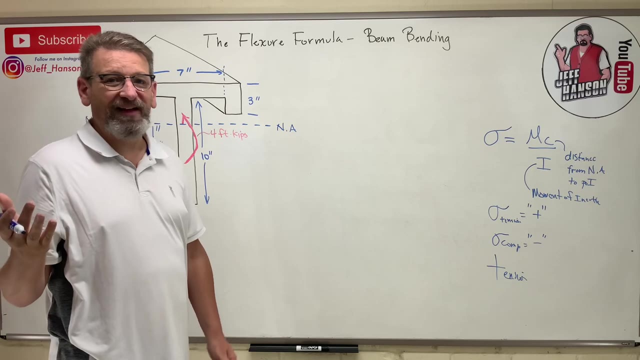 one. if the neutral axis is in compression, you're going to have a negative value, okay. so if that axis is important, we should probably find that right. so where, oh where, is that neutral axis? okay, which also you can also call that the centroidal axis. well, that sounds like we're gonna have to calculate a centroid, and that's exactly what. 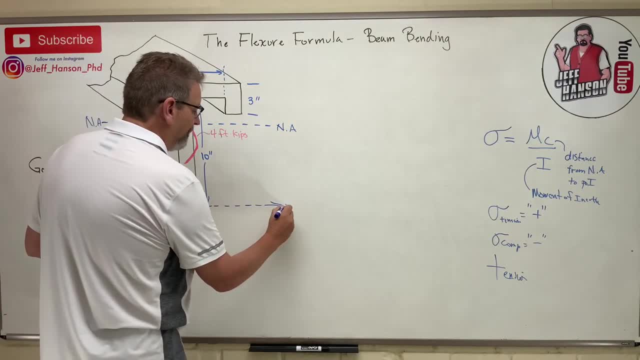 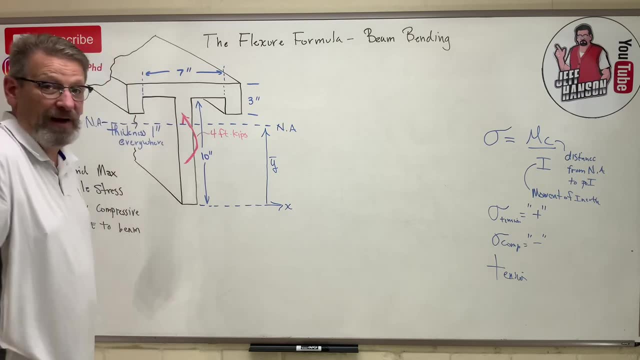 we're gonna do. i'm gonna make the bottom of my part my datum. i'm gonna call that x and what i need to find is where does that neutral axis live? and i'm going to call that y bar bar. So I'm looking for Y bar for this shape. Let's do a little statics 101 here, okay. So let's make. 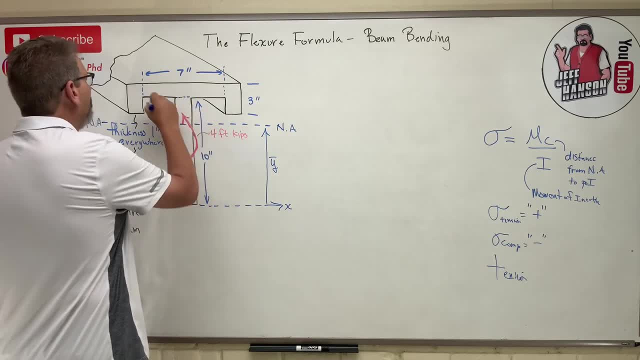 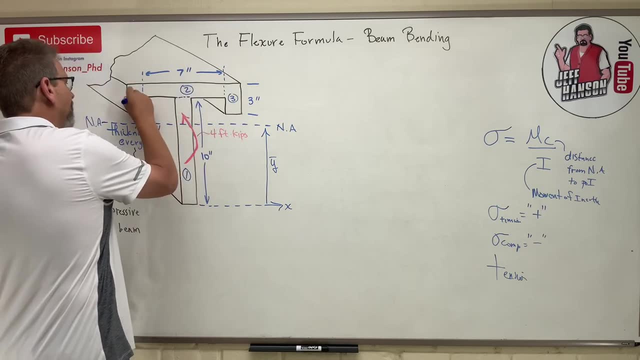 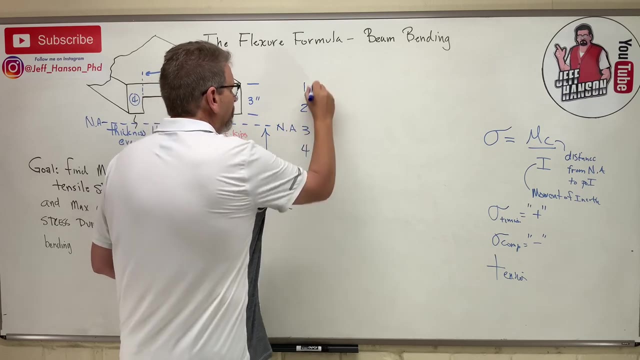 a let's break this into component parts here. I'll call this a piece one, piece two, piece three, piece four. How's that Okay? so here we go. Let's do this: One, two, three, four, Okay, and then what? 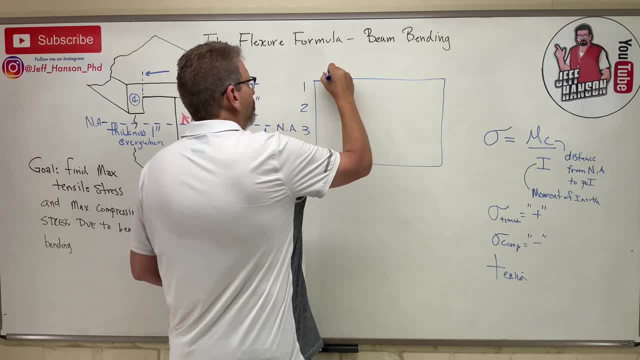 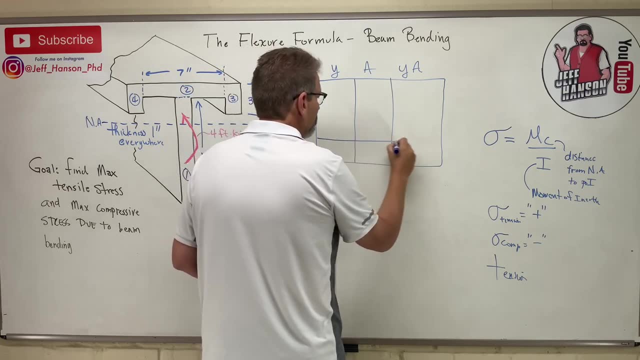 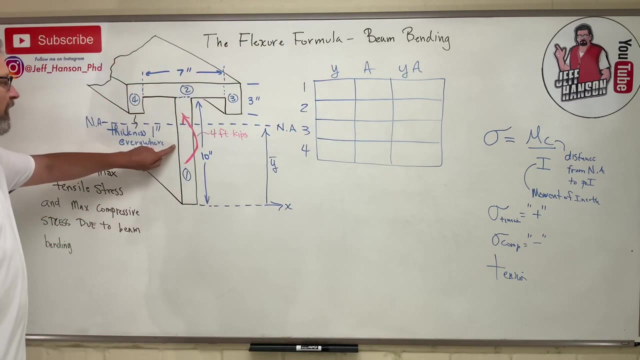 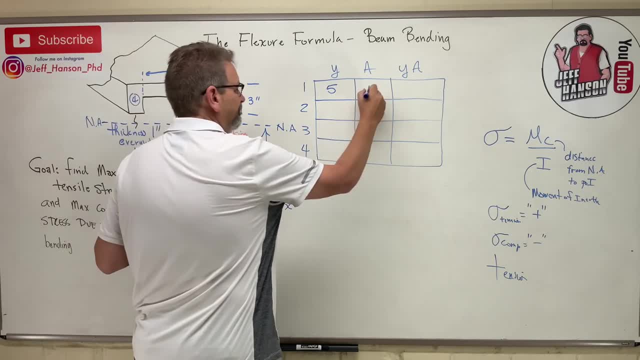 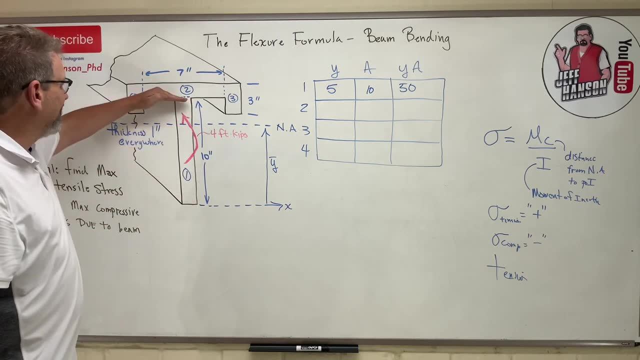 one inch right. So one by 10 is 10.. Which would make that 50.. I just did that in my head. Okay, Y bar for shape two. I'm going to go 10 to get up here, and then the Y bar lives at half of one. So how about 10.5?? 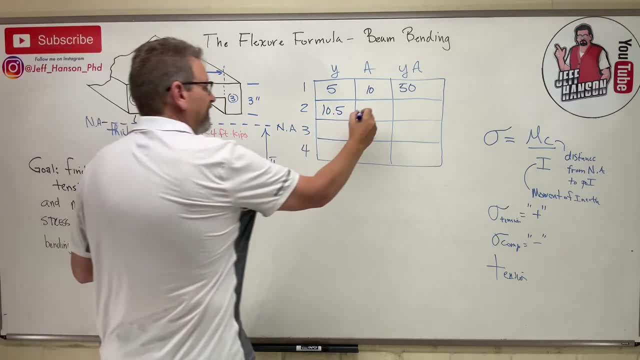 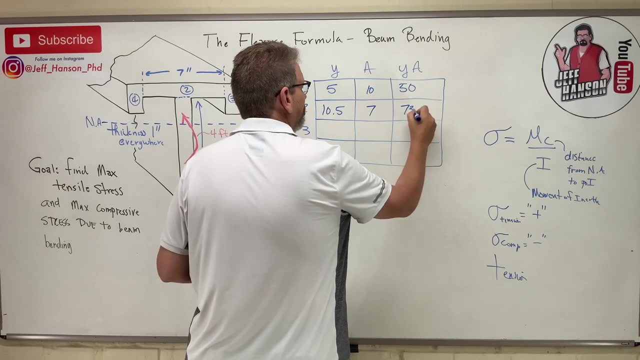 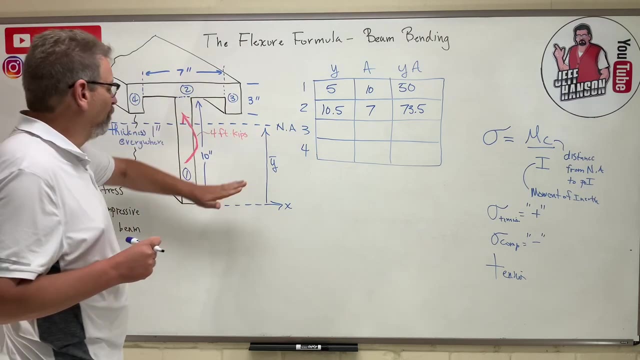 And the area is seven by one, That's seven. Okay, what is that? That's 70 plus 3.5.. 73.5, right. So for piece number three, let's find Y bar, Let's go all the way to the top of the part, So that's. 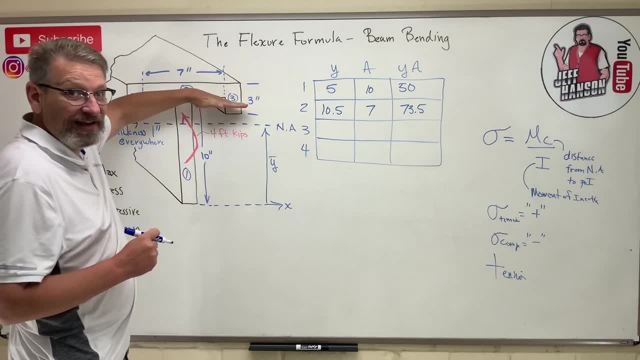 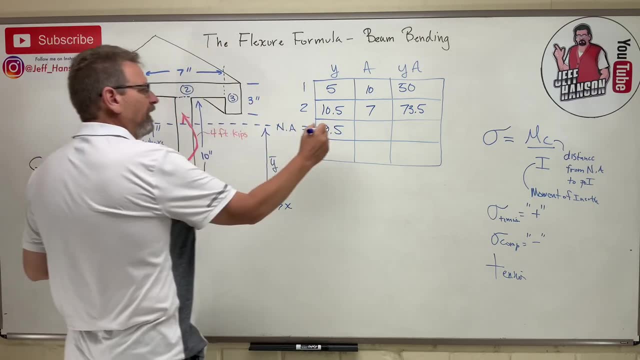 10 plus one, That's 11.. And then come back an inch and a half, So that puts us at nine and a half, doesn't it? And the area three by one, So that's three. Let's see, Nine times three is 27,. 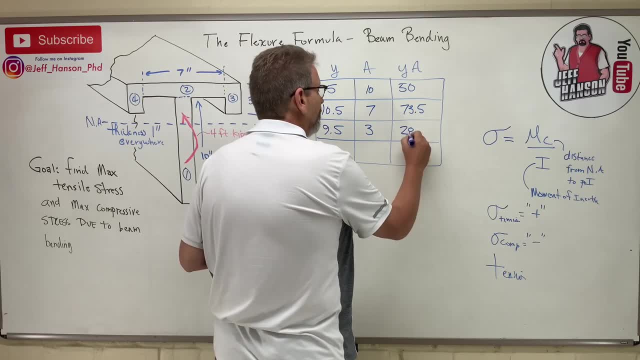 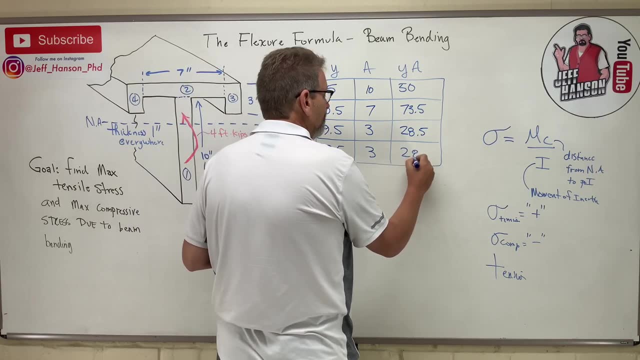 plus 1.5 is 28.5.. And piece number four also 9.5.. Three, 28.5.. Okay, so now we just need to add up our sum of the A's, So that's 17.23.. 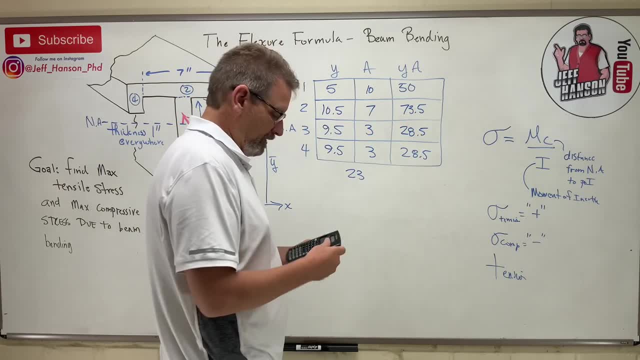 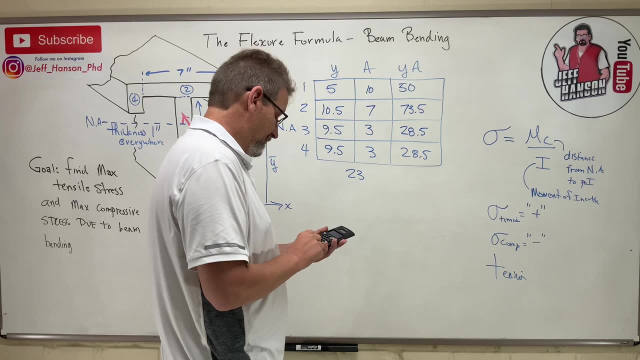 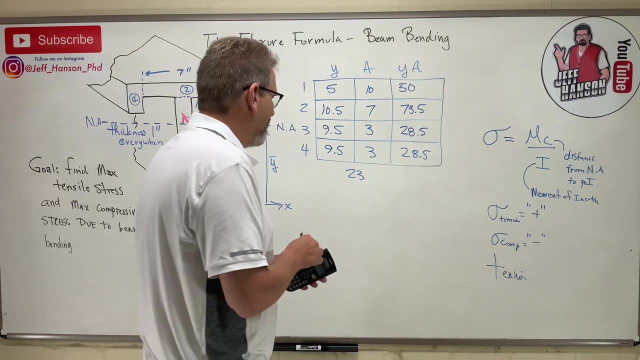 Sum of the Y A's. I'm going to have to do that one in my calculator. I don't have to, but I'm going to 50 plus 73.5 plus 28.5 times two 180.5.. 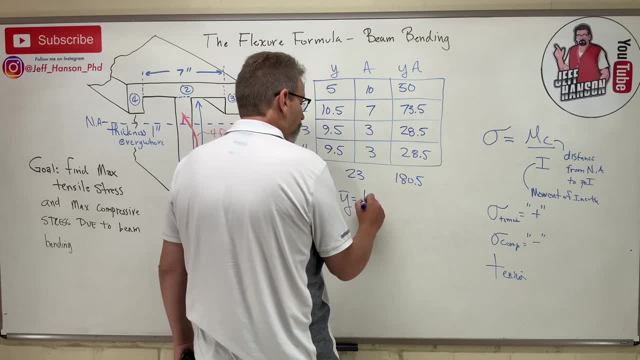 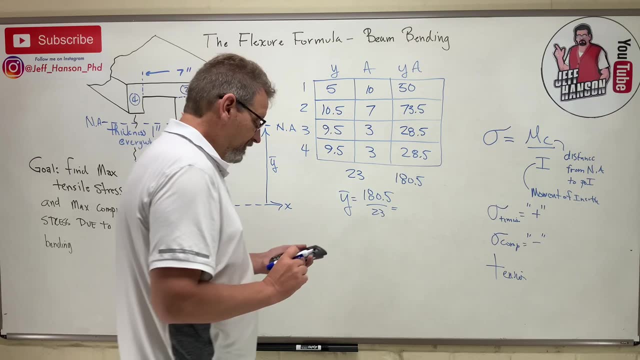 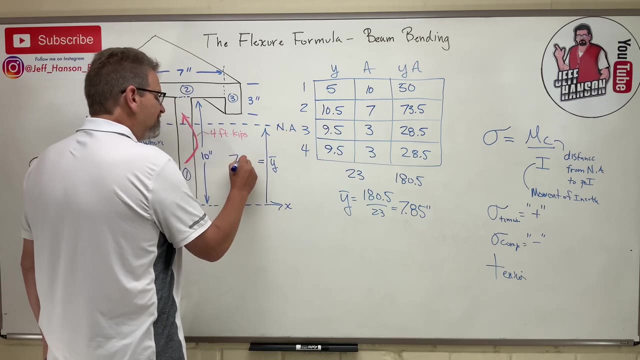 So Y bar is equal to 180.5 divided by 23,, which is divided by 23,, 7.85.. So this Y bar here, 7.85 inches. Okay, so it tells us where the neutral axis is from the bottom of. 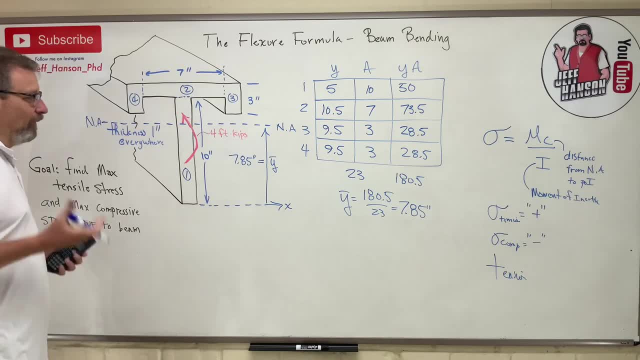 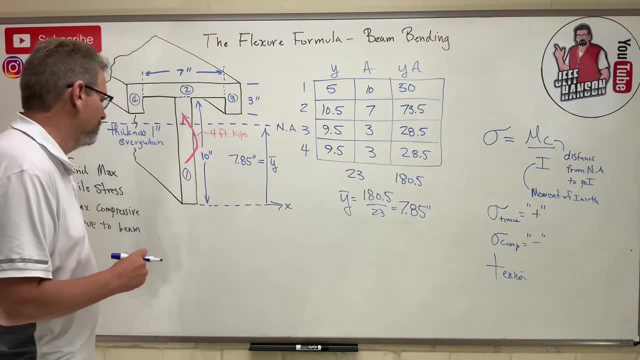 the part: Okay. well, why did we need that? Well, we need that to calculate this guy right here. then we need to calculate this guy right here. So we need to calculate this guy right here. the area moment of inertia. Okay, we're going to have to use the parallel axis theorem. 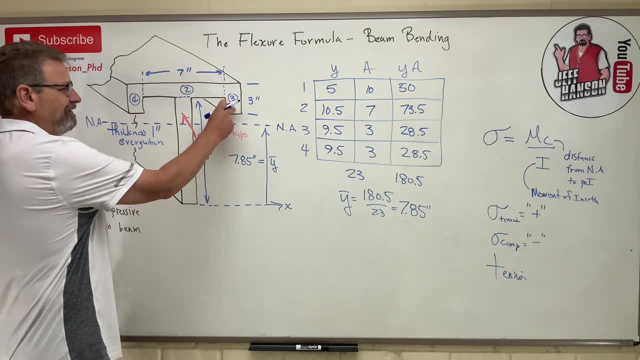 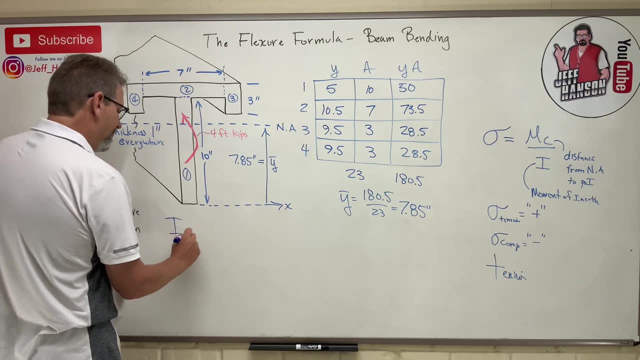 We got one, two, three. I can multiply this guy by times two, since there's two of them, So three parts. So here we go, I X. we'll call it I X prime. That's the moment of inertia about the. 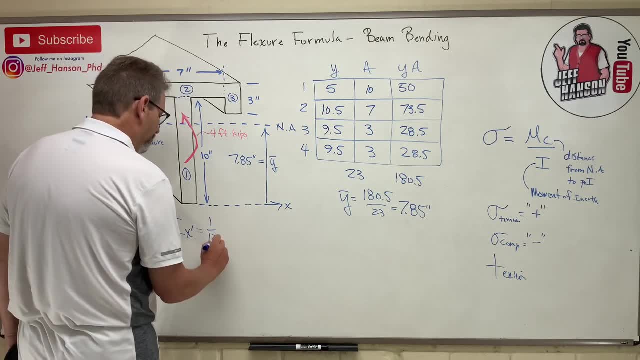 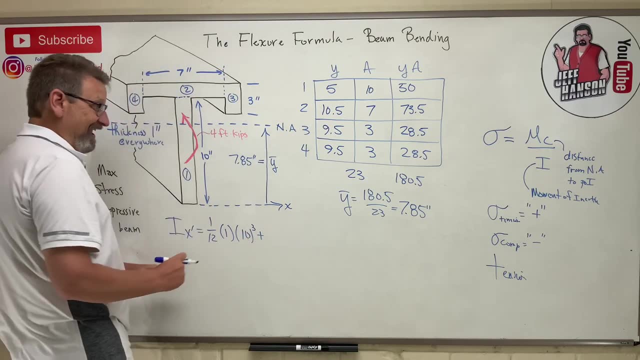 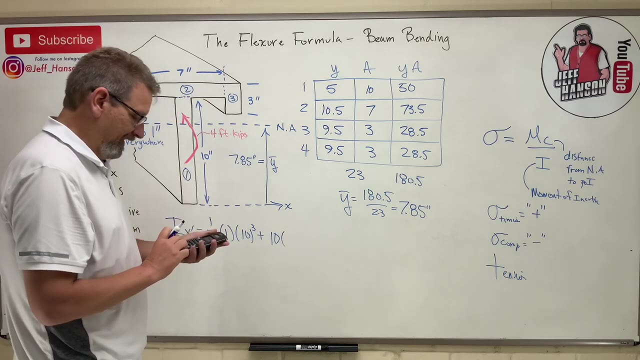 neutral axis. Okay so piece number one. one twelfth, the base one times the height, 10 cubed plus A. Remember A, B squared right, So A is 10.. And then what is D? D is 7.85 minus. 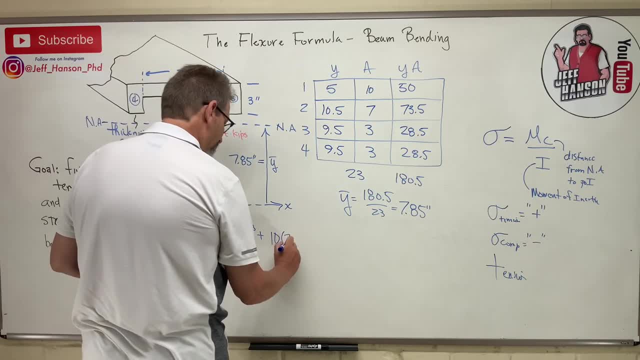 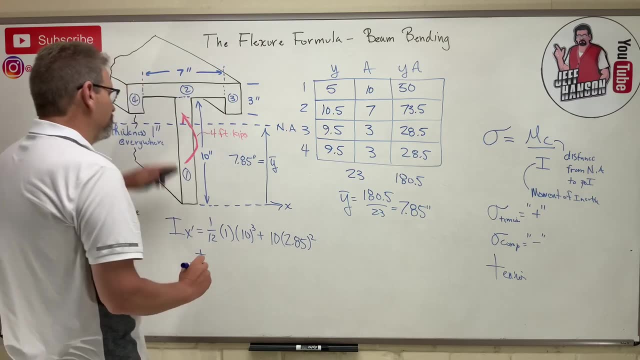 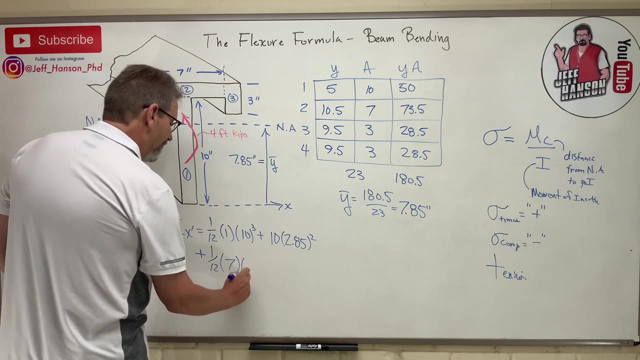 well, minus five. Well, I'm going to put that in my calculator, It's 2.85.. Okay, there's piece number one plus piece number two. this guy one twelfth. the base is seven, The height is one. 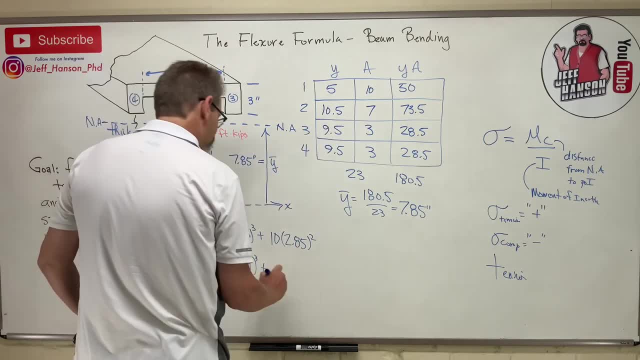 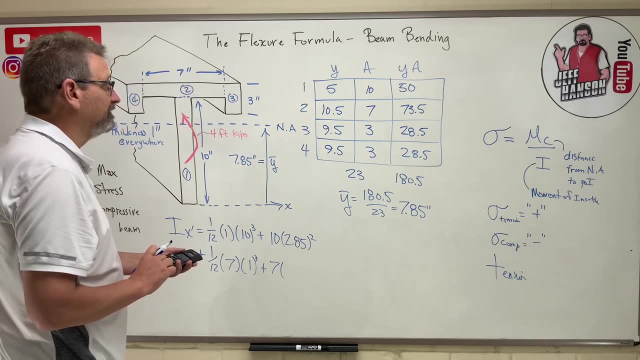 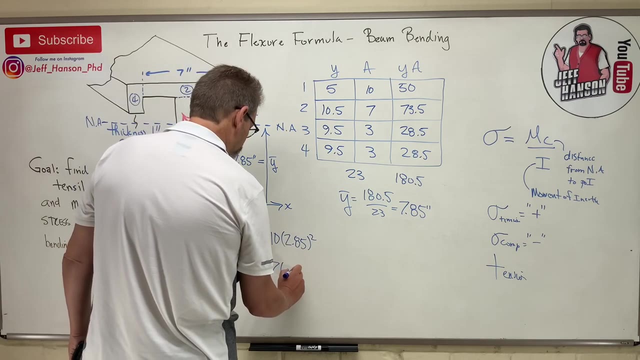 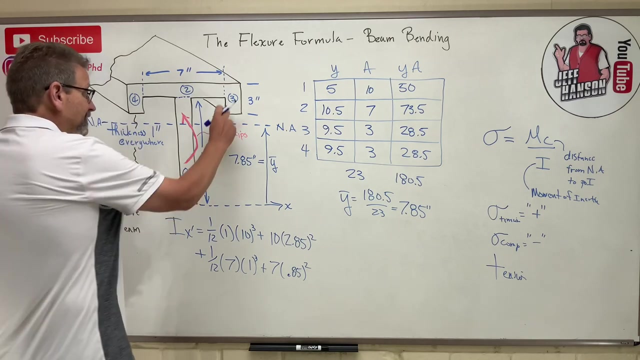 plus, the area is seven And D is 7.85. minus what seven, right, 0.85.. Okay, And then finally, these two pieces here, right? So I'm going to do this, I'm going to do. 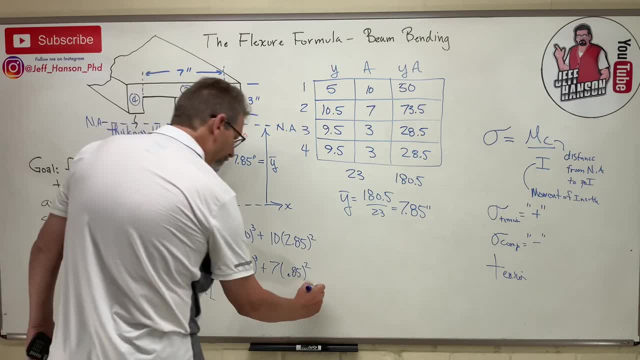 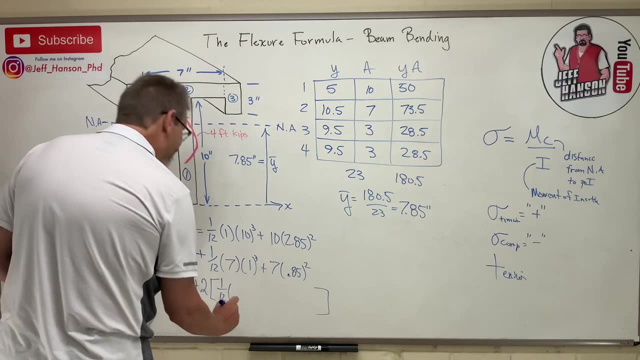 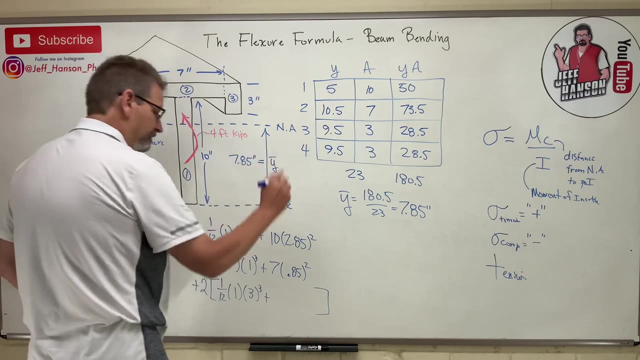 plus two times, and I'm going to do the whole thing right Because there's two of these pieces here. So one twelfth the base, one the height, three plus the area, three times D, What is D? 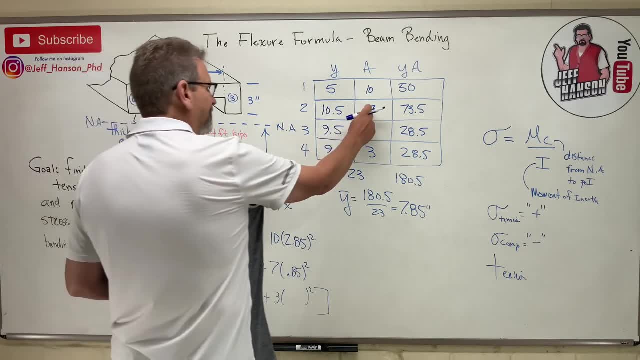 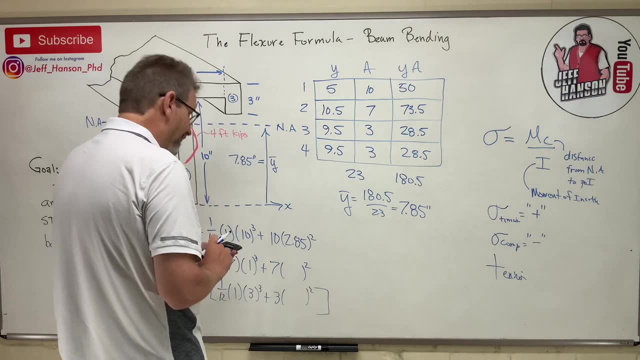 D. Oh, I didn't do that right. Wait, I used seven. I shouldn't have used seven. I should have used 10.5.. Oh, that was going to be bad, Wasn't it? 7.85 minus 10.5.. That should have been 2.65.. 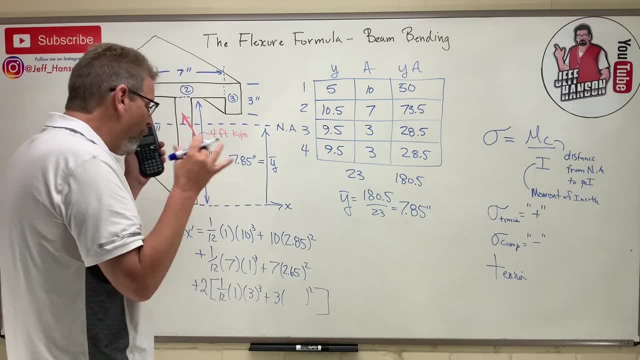 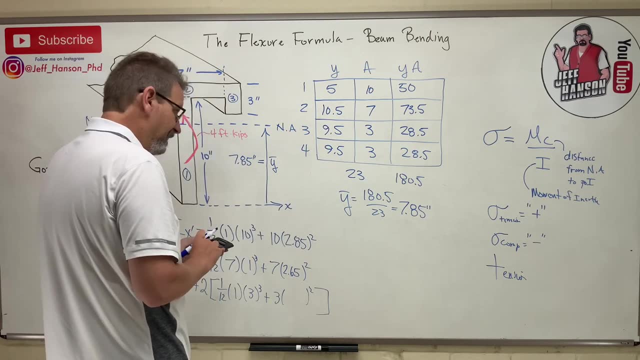 I'm glad y'all caught that Y'all were probably going: oh no, it's wrong, I got it, I got it, We're all good. So 7.85 minus 9.5 is 1.65.. 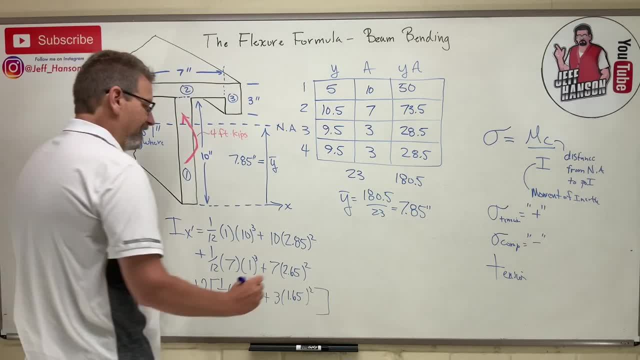 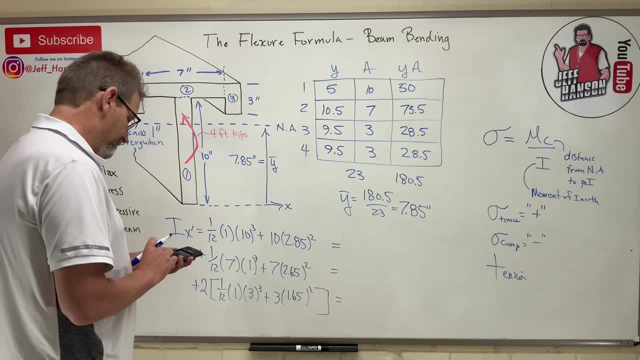 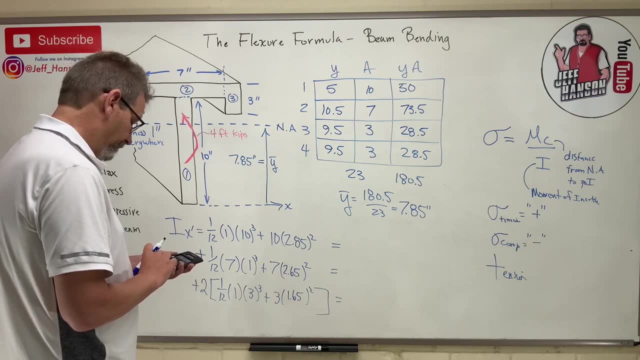 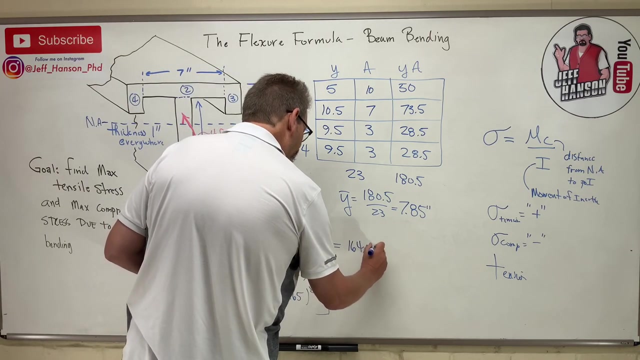 then add all those together. Okay. So what is that? 10 cubed divided by 12 plus 10 times 2.885 squared equals 164.56.. Okay, And these are going to be inches to the fourth, aren't they? 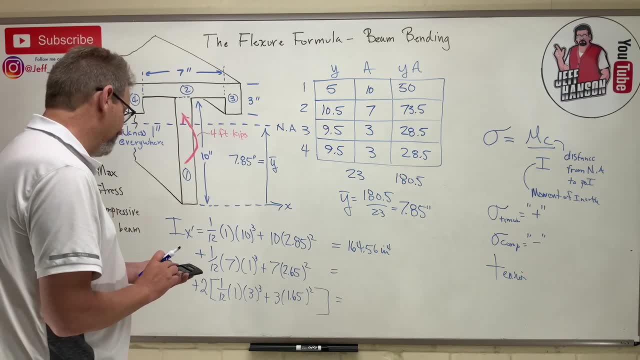 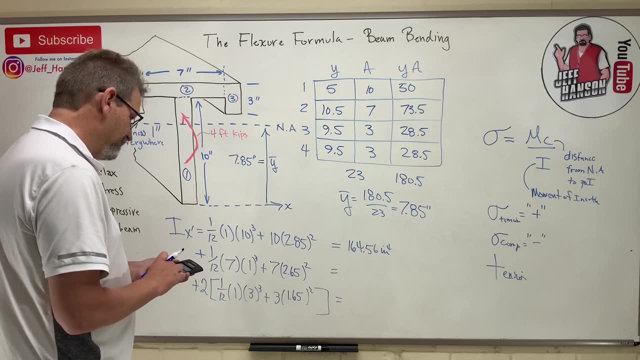 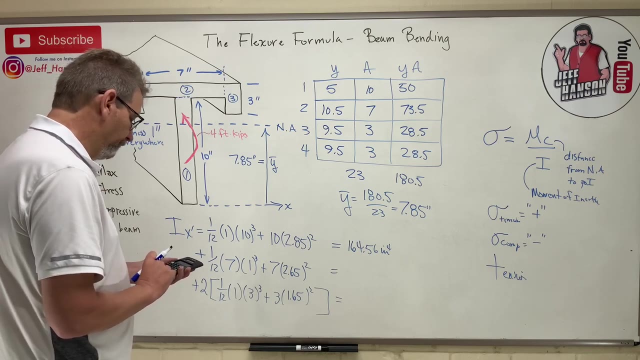 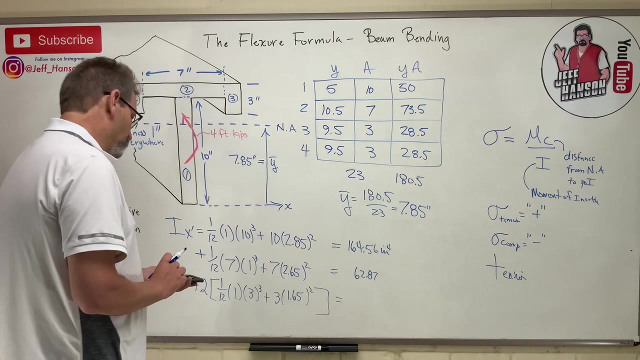 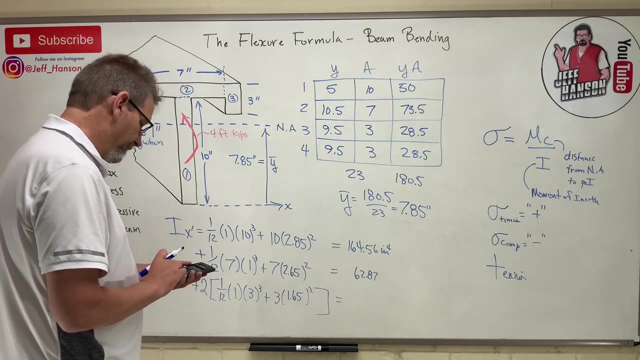 Okay, So the next one is going to be 7 divided by 12 plus 7 times 2.65, squared equals 62.86.. And the last one down there is going to be 3 cubed divided by 12 plus 3 times 1.65. 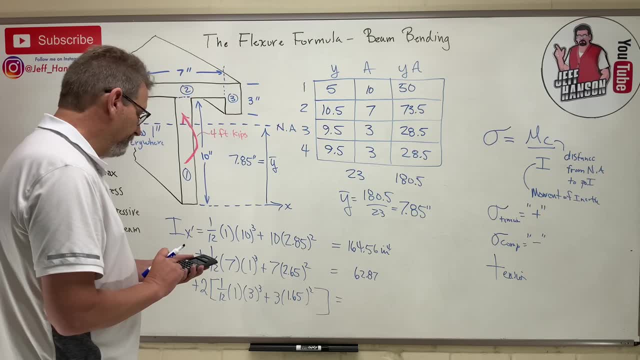 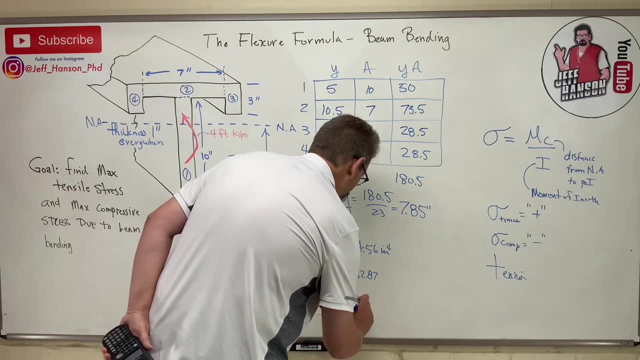 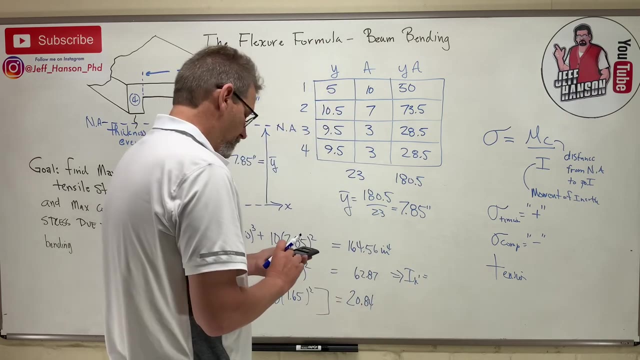 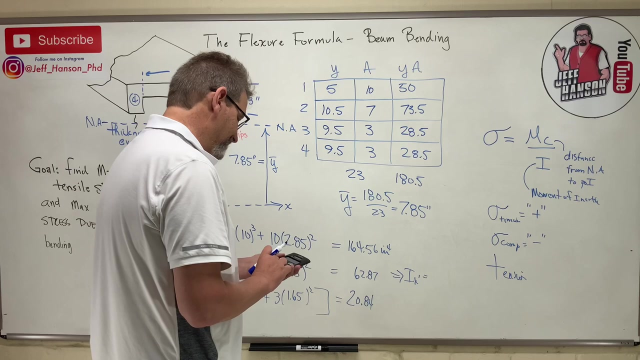 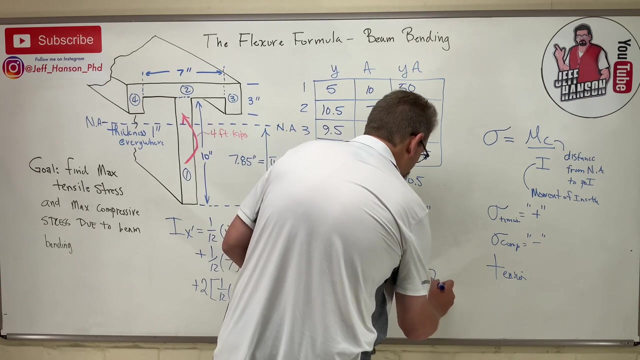 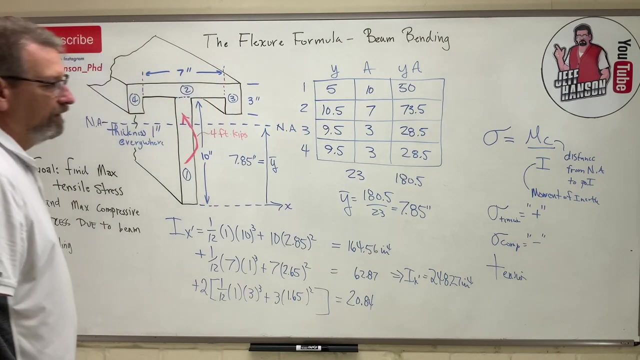 squared equals 10.41.. And then times 2 is 20.84.. So therefore, I x prime is equal to plus 62.87 plus 164.56.. I get 248.27.. Okay, Inches to the fourth. So what's left to do? Well, I'll tell you what's left to do. All we got. 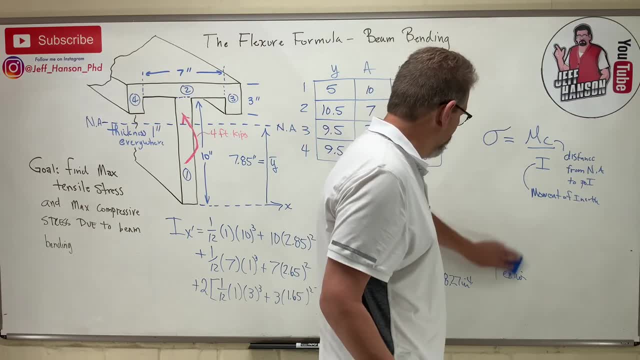 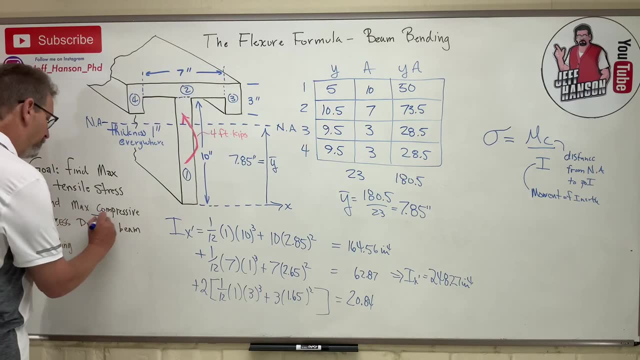 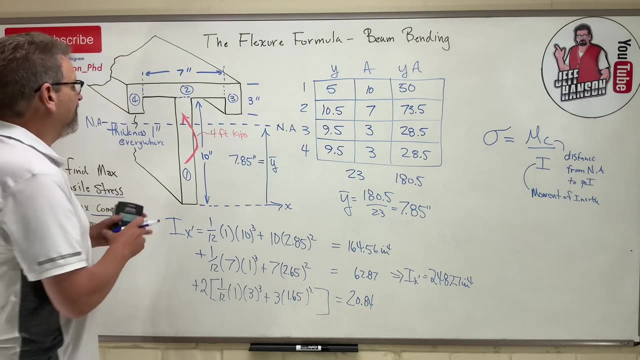 to do is use our little equation- we learned today the flexure formula- to solve this. Okay, So there's two. they asked us about The maximum compressive and the maximum tensile. There it is Okay. So again, if we have this right, the compression is going to be on the 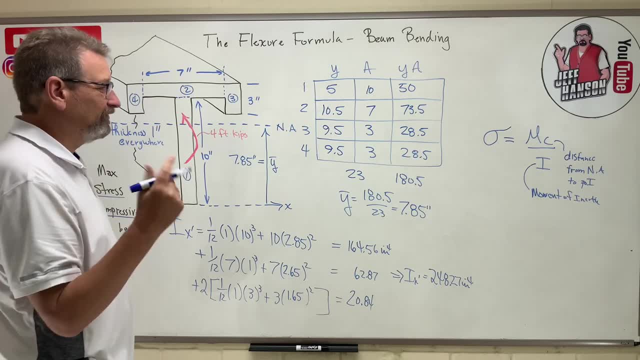 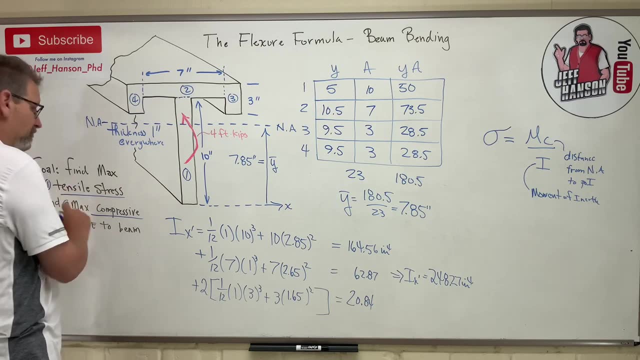 top. So what is C? Let's do. let's do the compress, Let's do tensile first. This is the first one. Okay, Number one, Number two: Okay. So tensile. If I bend it like this, tensile is on the bottom. So I'm interested. 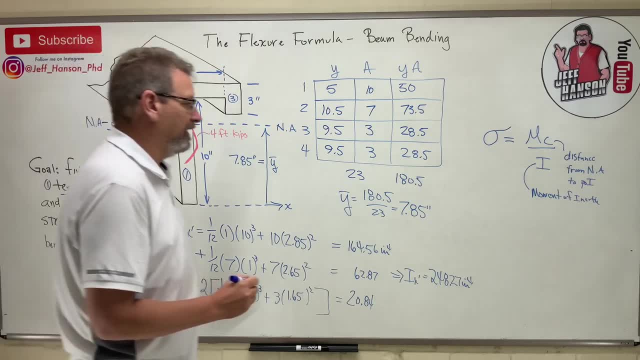 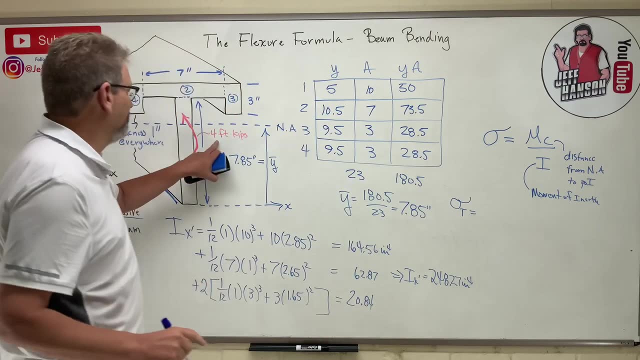 on these fibers at the very bottom of the part. Okay, So, here we go. Sigma, I call it. T for tension is equal to M. M is given Four-foot kips. Now be careful of mixed units here. Okay So four. 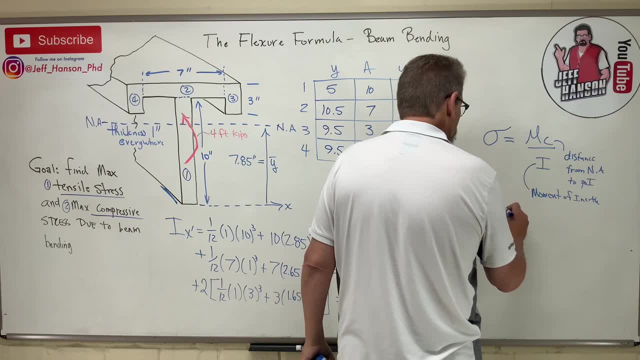 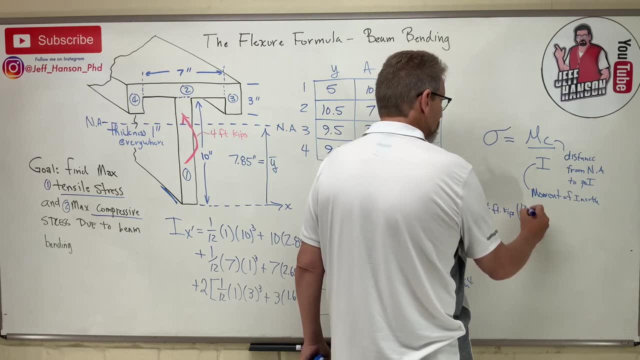 foot tips. okay. So I'm going to get rid of that foot right there. I'm going to put him on the bottom and that's 12 inches, right. So then my feet cancel out. Okay. so there's M times C. 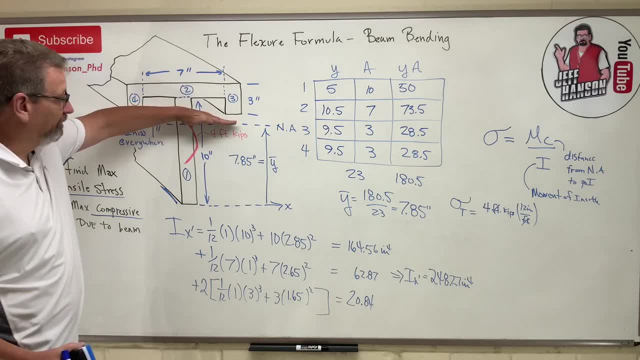 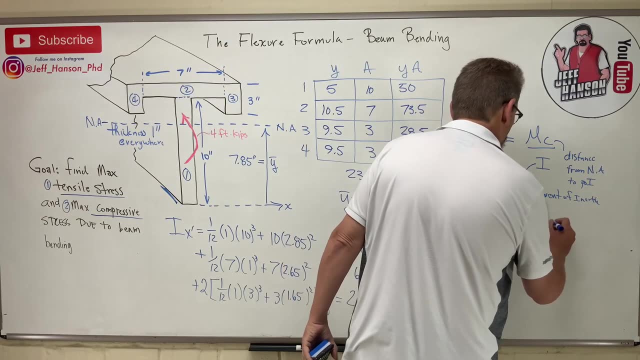 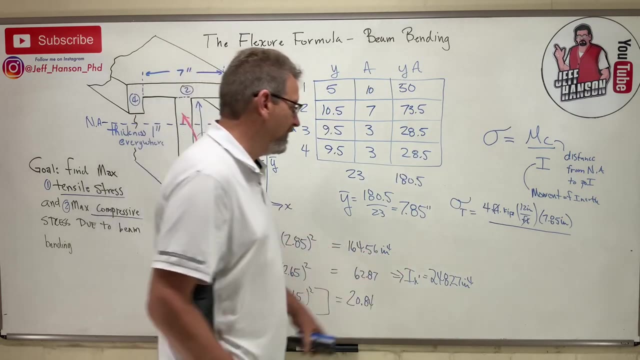 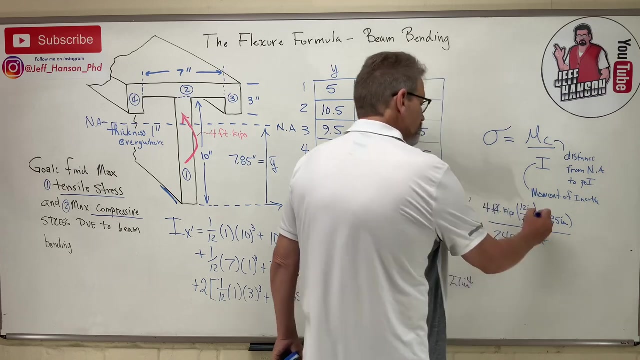 Well, C is the distance from the neutral axis to the point of interest and for tension I'm interested in down on the bottom. So C is going to be 7.85, okay- Divided by I, which we just calculated right here: 248.27 inches to the fourth right. So two of the inches cancel out two. 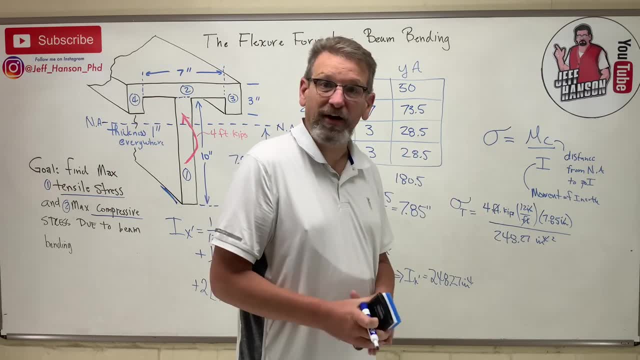 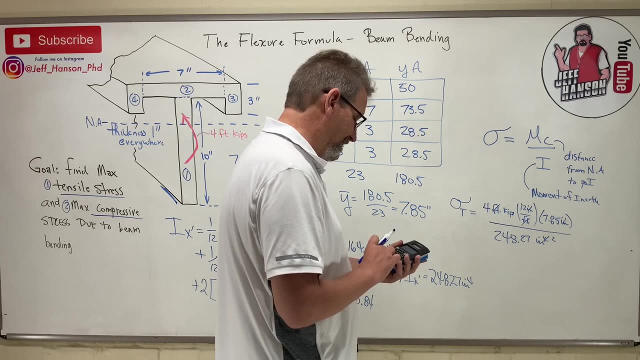 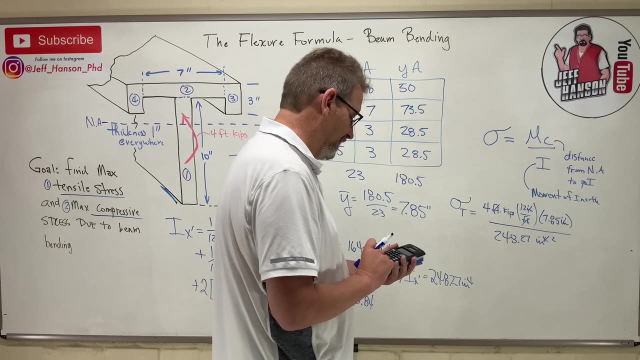 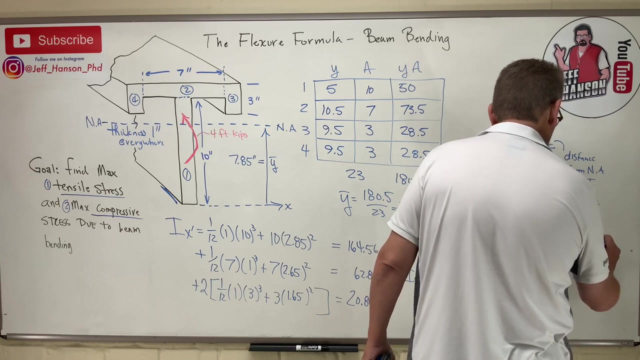 of those inches and it's going to leave me with kips per inch squared, which is KSI, right. So here we go: 48 times 7.85- equals. divided by 248.27 equals: 1.52 KSI. okay, 1.52 KSI okay. 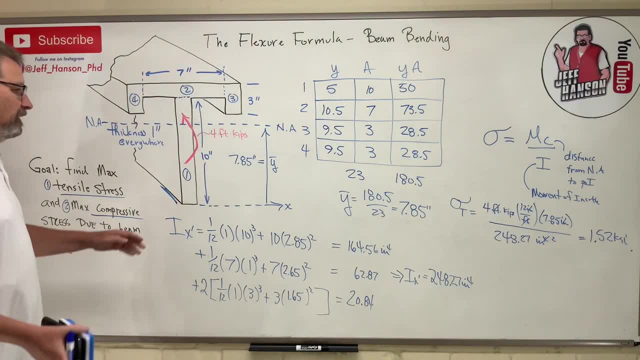 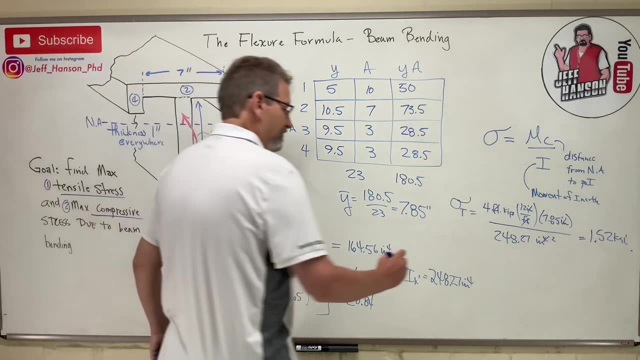 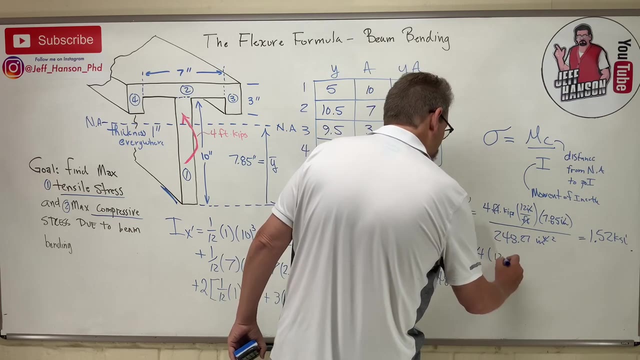 There's the maximum value of stress for tension. So what is the maximum component? Compressive stress? That's going to be on the top of the beam, okay, So what is that going to be? Sigma compression is equal to same moment 4 times 12,, okay, Times C. Oh, I bet C is different. 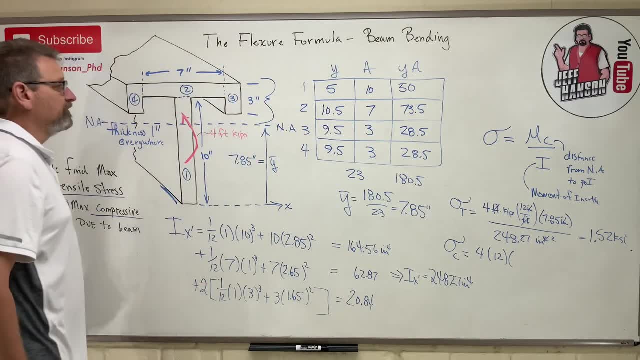 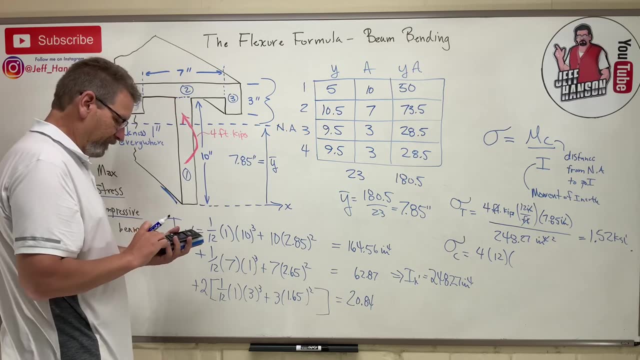 because C is now this distance here. So how far is that? Well, the whole part is 11 tall, So from here to here is 7.85.. So 11 minus 7.85, that means that this must be 3.1,. 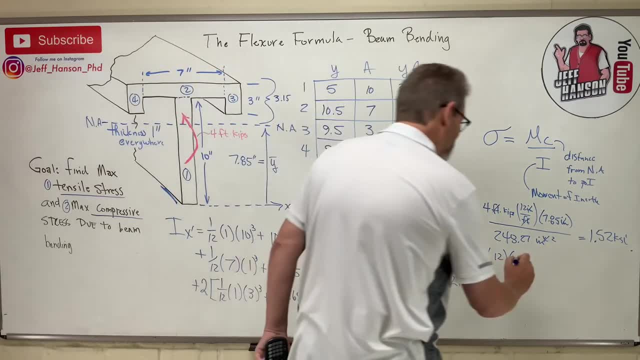 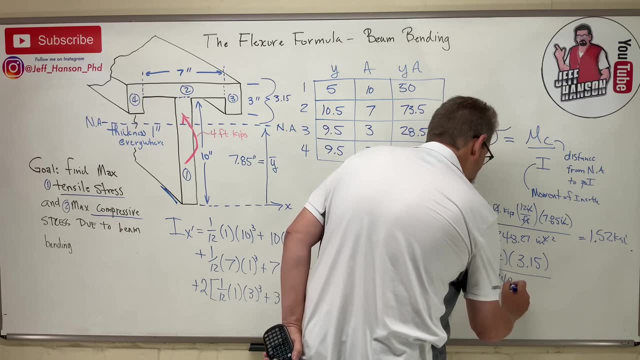 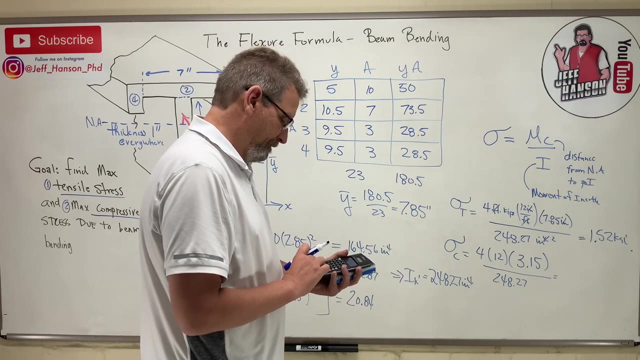 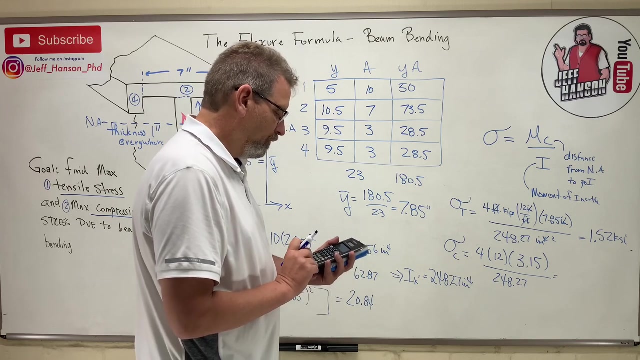 right, And that's my C for compression: 3.15.. Divided by the same, I 248.27.. Let's see what we get here: 48 times 3.15, divided by 248.27, equals 0.609 KSI. 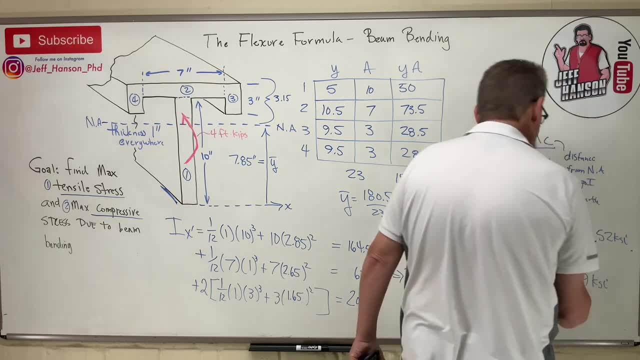 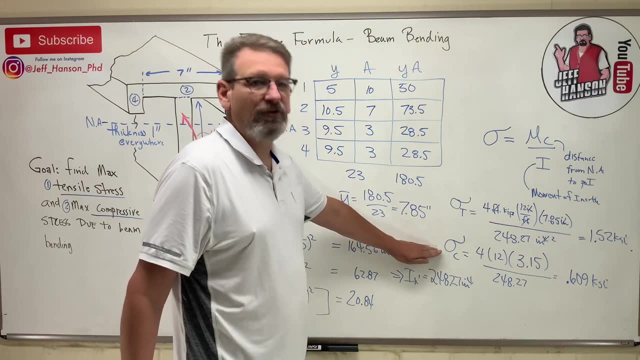 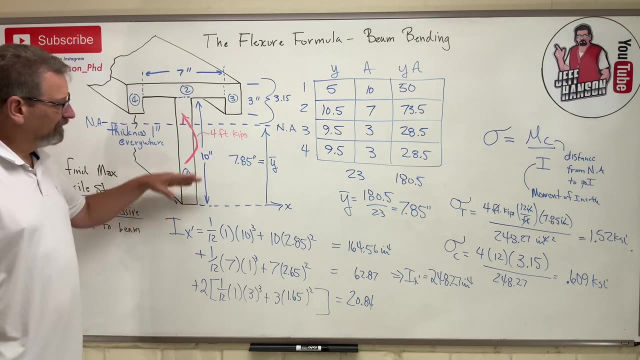 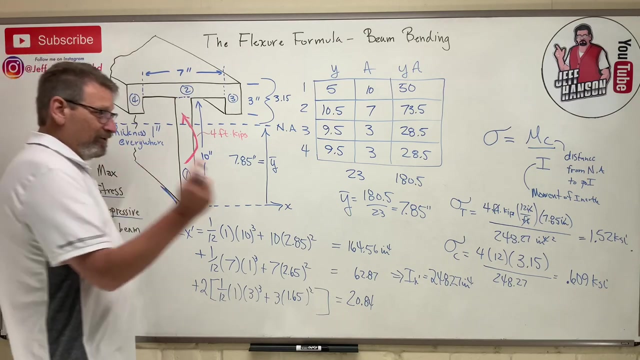 Okay, And there you go. So there's the maximum tensile stress due to bending, The maximum compressive stress due to bending. So, step one, find your neutral axis. Step two, calculate your moment of inertia and then get your distance to the point of interest and go to town Units. 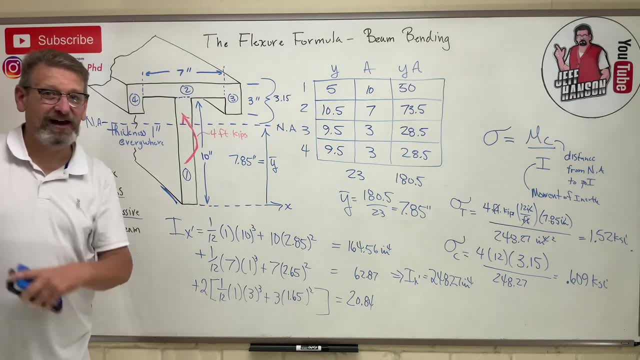 units, units. Be careful about your units on this. okay, I'll see you next time, gang. Bye-bye.